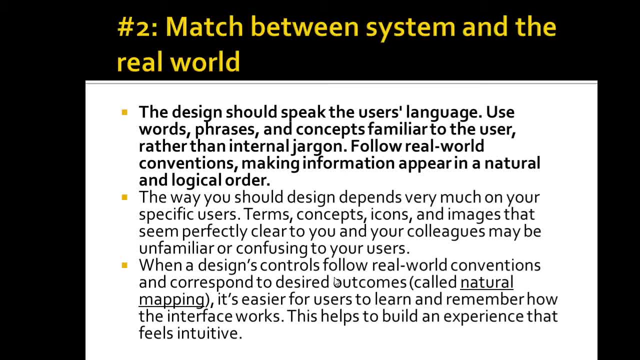 order. the way you should design depends very much on your specific users. terms, concepts, icons and images that seem perfectly clear to you and your colleagues may be unfamiliar or confusing to your users. when it designs, controls follow real world conventions and correspond to desired outcomes. called natural mapping, it's easier for users to learn and remember how the interface works. 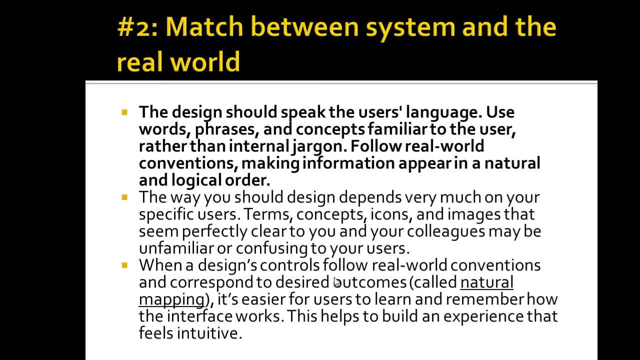 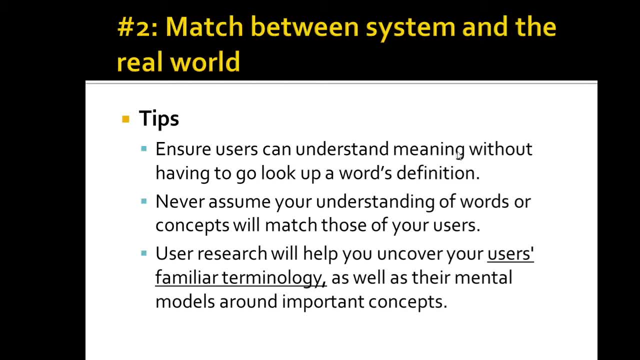 this helps to build an experience that feels. intuitive tips ensure users can understand meaning without having to go look up a word's definition. never assume you understanding. your understanding of words or concepts will match those of your users. user research will help you uncover your users familiar terminology, as well as their mental models around important concepts. 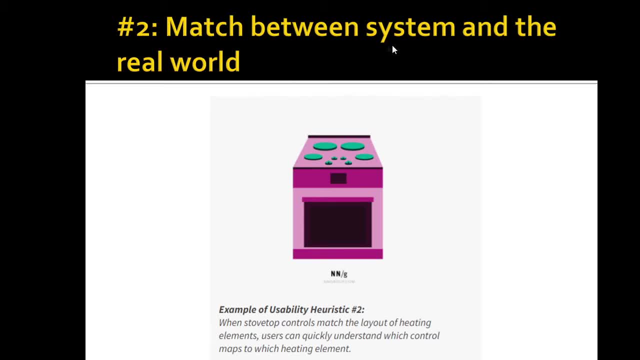 so here's an example of matching the the system and the real world. so when oval, when soap stop controls, so so these are stove stop controls- match the layout of hitting elements. that's why this is for this and this control is for that, this one's for this and for this. so it matches the layout so users can quickly understand. 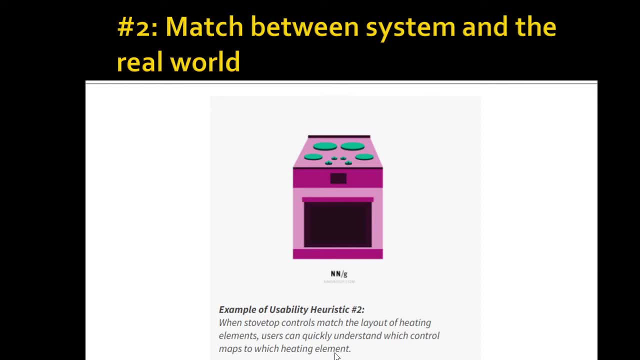 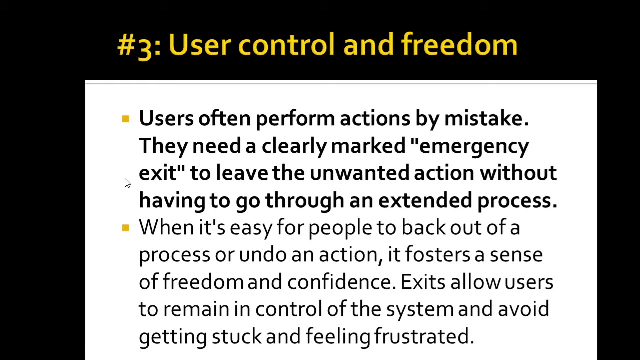 which control maps to which heating element. so rather than having this maybe in straight line, this one is better because it matches the layout of the heating element. so that's an example of applying this rule. number three: user controls and freedom. users often perform actions by mistake. they need a clearly marked emergency exit to leave the unwanted action without having to go. 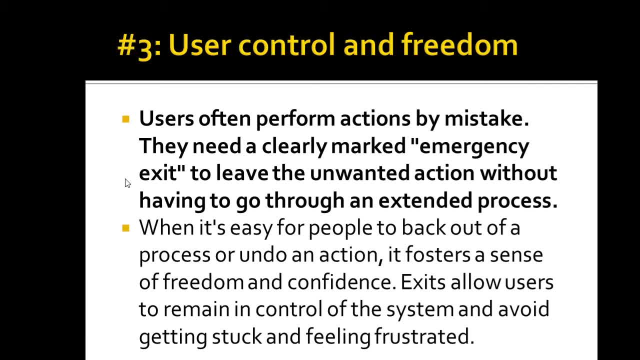 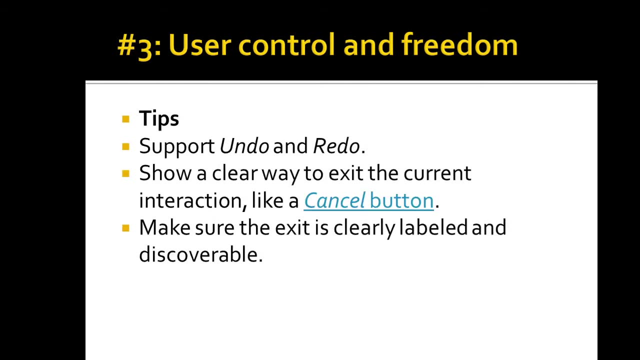 through an extended process. when it's easy for people to back out of a process or undo an action, it fosters a sense of freedom and confidence. exits allow users to remain in control of the system and avoid getting stuck and feeling frustrated. tips, support and do and redo, so that will, of course, make it easy for users to get back. 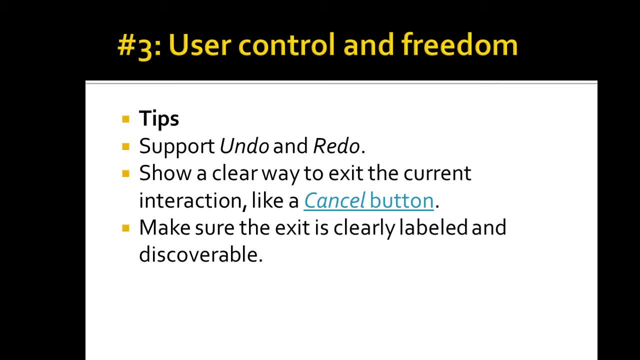 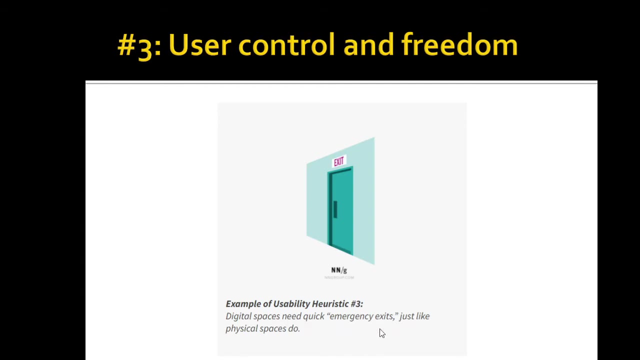 out of a process and do our mistakes and maybe redo if it is okay. show a clear way to exit the current interaction, like a cancel button, and make sure the exit is clearly labeled and discoverable. so here's an example. so again, digital spaces needs quick emergency exit, just like physical spaces do. 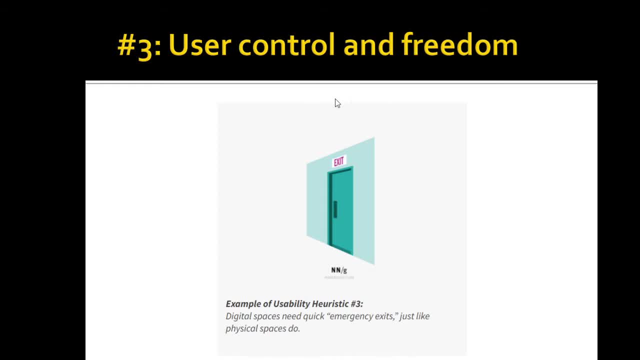 so for us, the, it will be um nice to know if you know that there are emerging emergency exits in a building, so in case of emergency, you know where to go out. but the same is true with software or design, so there should be a way for users to get out of. 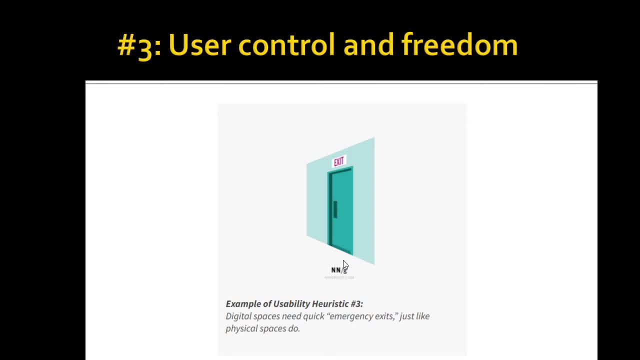 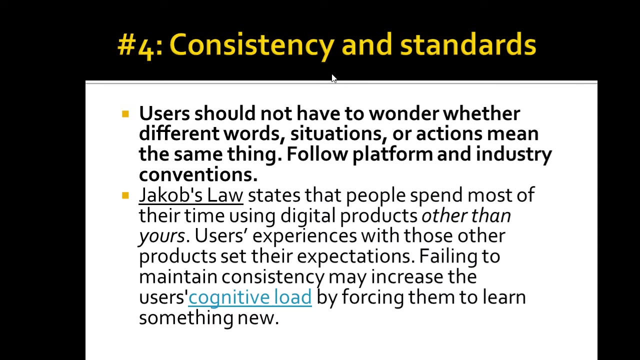 whatever they are in, so like cancelled buttons, or maybe you committed a mistake. you can undo your errors, so this is about it. Don't forget to like this video and share it with your friends. Thanks, опять na ke网 Paris. user control and freedom. the number four: consistency and standards. users should 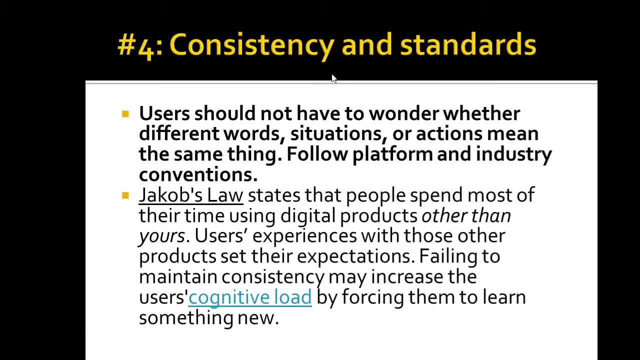 not have to wonder whether different words, situations or actions mean the same thing. you have to follow platform and industry conventions. Jacob's law state that people spend most of their time using digital products other than yours, so there they might be using other product than what you are using, so 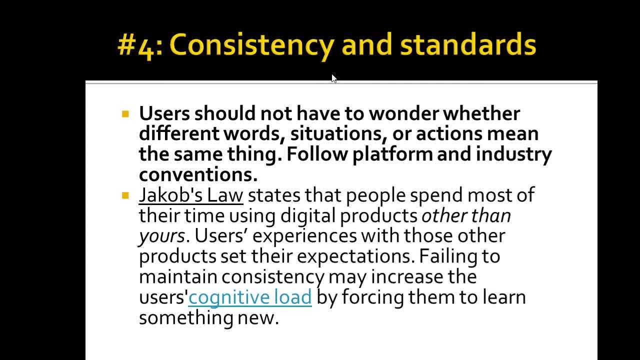 users experiences with those other products set their expectations. failing to maintain consistency may increase the users committee load by forcing them to learn something new, so don't think that what you are using is also what they are using. so, again, you have to follow standards and to be consistent so that you will not be increasing the 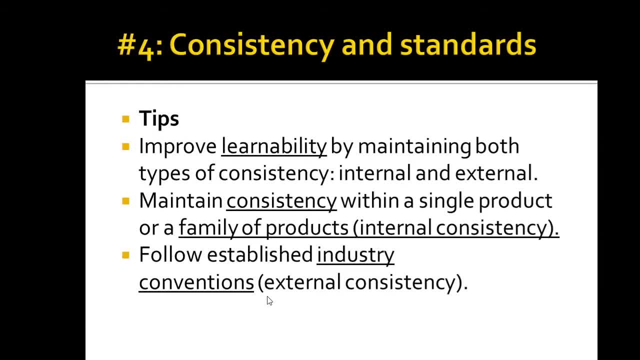 committee load of users. so here are some tips: improve learnability by maintaining both types of consistency, which are the internal and external consistency. maintaining consistency within a single product or a family of products is internal consistency. so if you have a product or you have a group of products, 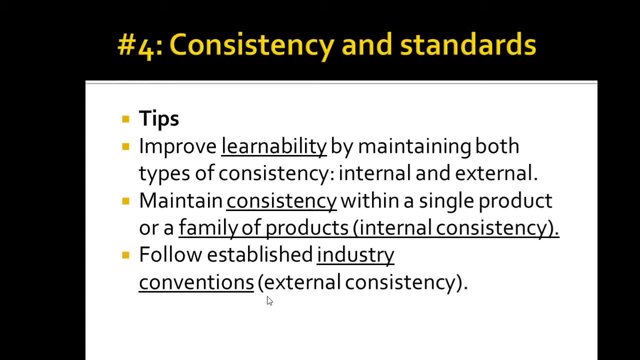 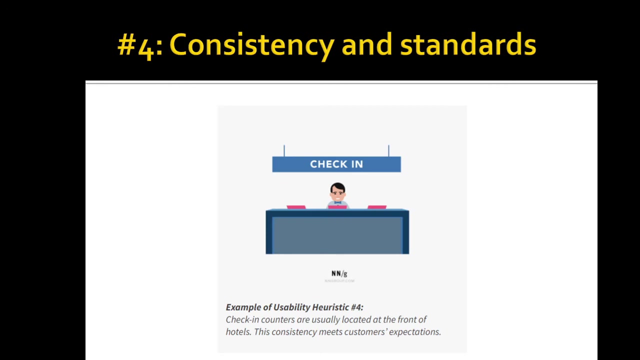 then there should be something consistent with these products or the external one, so이스 School of Maison 留 world map. see more links in the video description below. so you have to follow these conventions, especially if this is the acceptable convention. for example, visibility heuristic number four. check-in counters are usually located at the front of hotels. 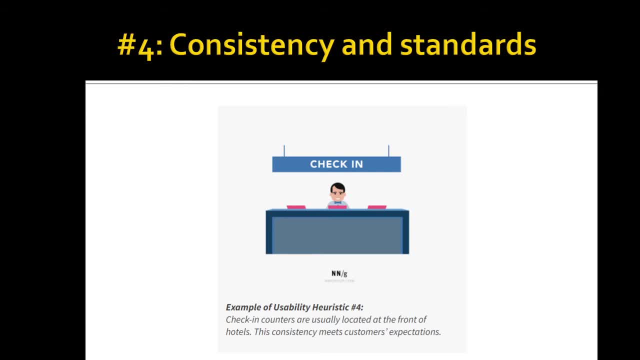 this consistency meets customers expectations. so if you are a customer, you would expect that the check-in counters will be at the front of the hotels, because that's the standard. so if you're going to arrange your, if you have a hotel, then you should place. you should always place your. 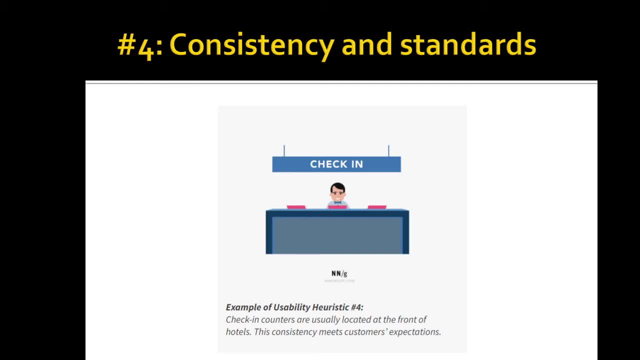 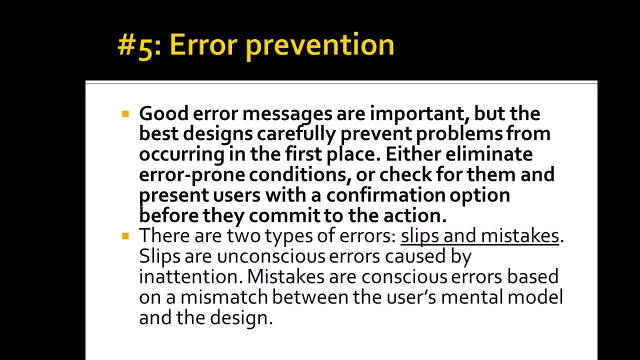 check-in counter at the front of hotels. so that's following the standards. number five, excuse me. number five is about error prevention. good error messages are important, but the best designs carefully prevent problems from occurring in the first place. so not just showing error messages, but we should prevent the occurrence of errors. 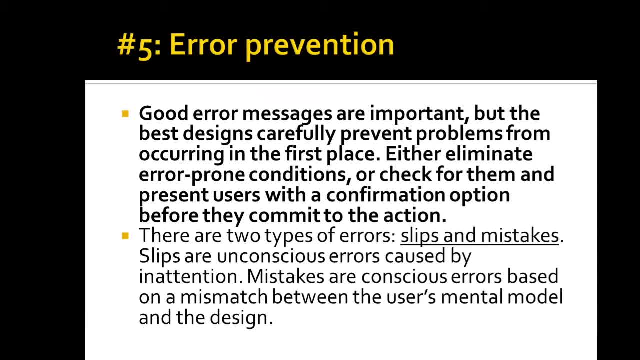 either eliminate error prone conditions or check for them and present users with the confirmation options before they commit to the actions. there are two types of errors: slips and mistakes. slips are unconscious errors caused by inattention, so mistakes are conscious errors based on a mismatch between the user's mental model and the design. so these are the different. 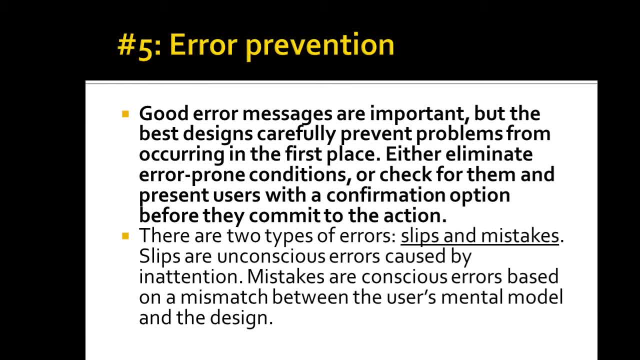 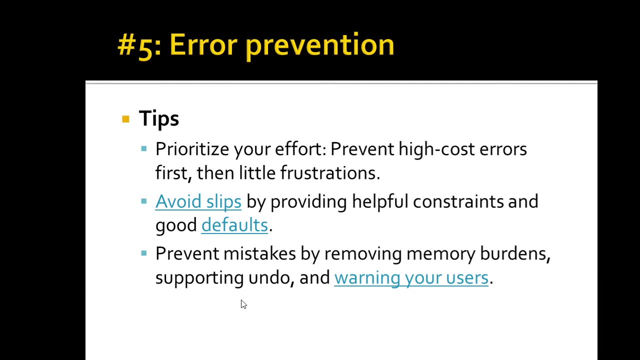 slip again. you're unconscious about it, but in mistake. you're conscious about it, but unfortunately what you know it's not um, it's not about uh, it's not much demand and the design. so, tips, prioritize your effort. prevent high cost errors first, then little frustrations. so if you're creating an, for example, if you're creating a, 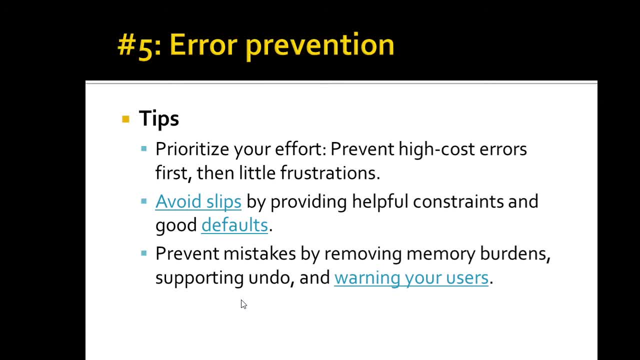 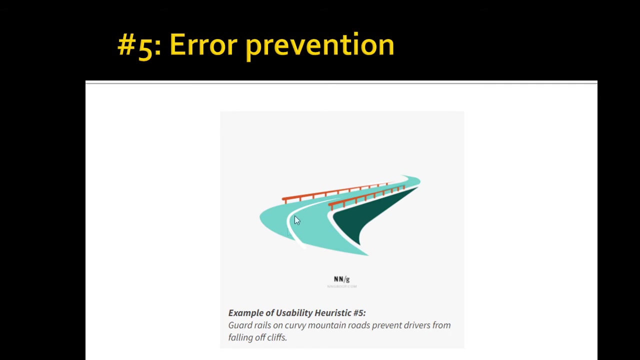 data entry program. so you should. your program should validate the entries of users first before you will be able to save. avoid slips by providing helpful constraints and good defaults. prevent mistakes by removing memory burdens, supporting undo and warning your users. so here's an example, a real-world example. 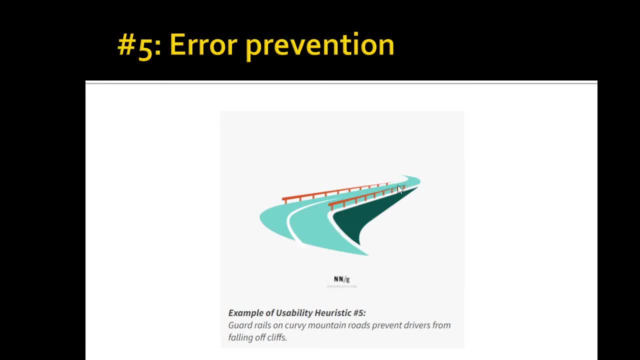 so guard rails. so these are the orange one on a curvy mountain road. prevent drivers from falling off clips. you have to prevent them from doing the error that is falling off clips, and what is used here are the guard rails. you have to prevent them from doing the error that is falling off clips, and what is used here are the guard rails. 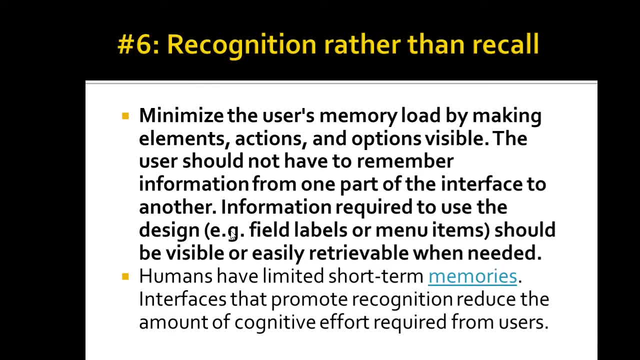 number six: recognition rather than recall. so minimize the user's memory load by making elements, action and options visible. the user should not have to remember information from one part of the interface to another. information required to use the design- example field labels or menu items- should be visible to air or easily retrievable when needed. 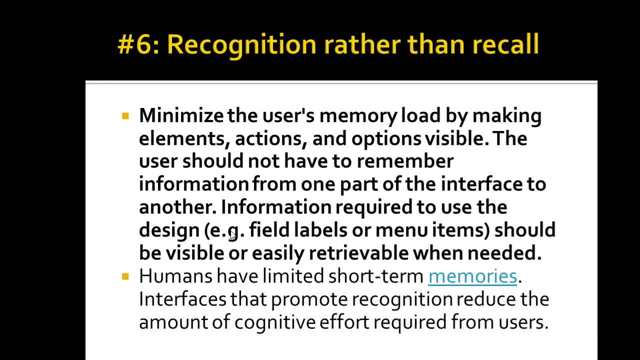 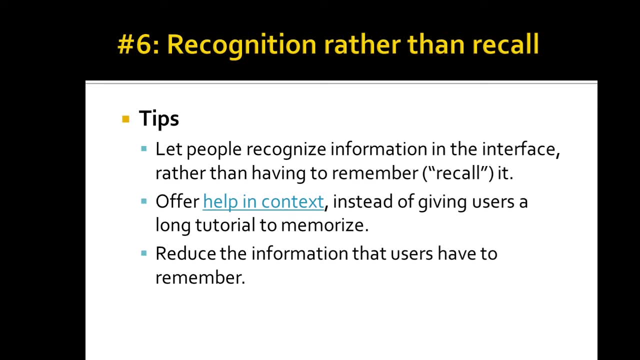 humans have limited short-term memories. interfaces that promote recognition reduce the amount of cognitive effort required from the users. tips: let people recognize information in the interface rather than having to remember or recall it or memorize it. offer help in context instead of giving users a long tutorial to. 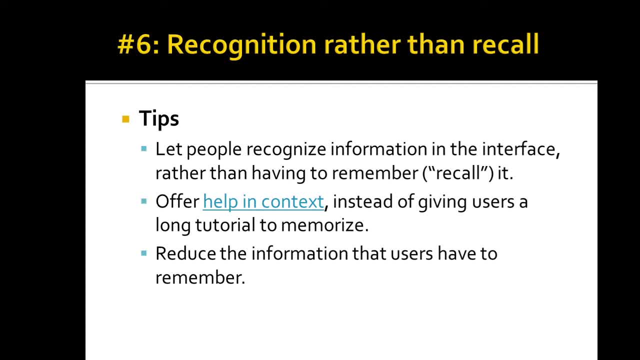 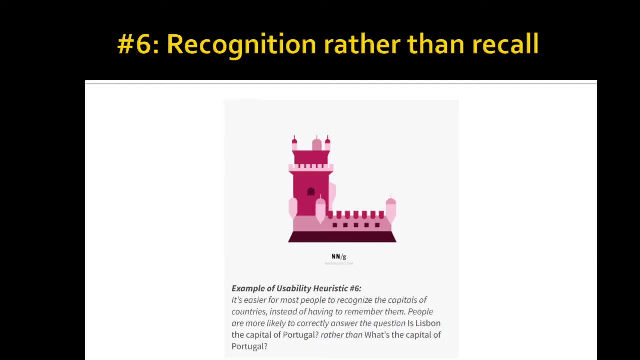 memorize reduce the information that users have to remember. so here's an example. so it's easier for most people to recognize the capitals of the countries instead of having to remember them. so how's that? here's an example. people are more likely to correctly answer the question: is lisbon, the capital of portugal, rather than this question? 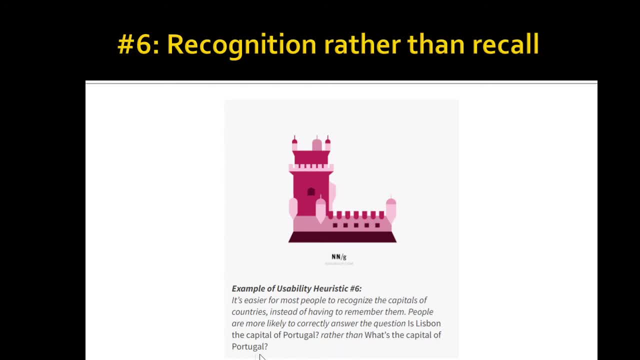 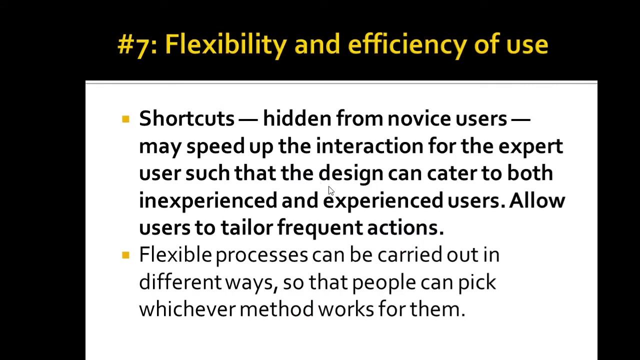 what's the capital of Portugal. because you say what's the capital of Portugal you have, you have to force the the people to recall. but here they are, just here to recognize: is this the capital or not? so it should be recognition rather than recall. number seven: flexibility and efficiency of use shortcuts. 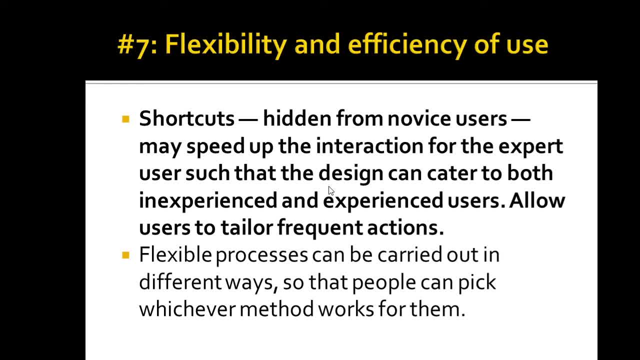 hidden from novice users may speed up the interaction for the expert user. sets that the design can cater to both inexperienced and experienced users. allow users to tailor frequent actions. flexible process can be carried out in different ways so that people can pick whichever method works for them. tips: 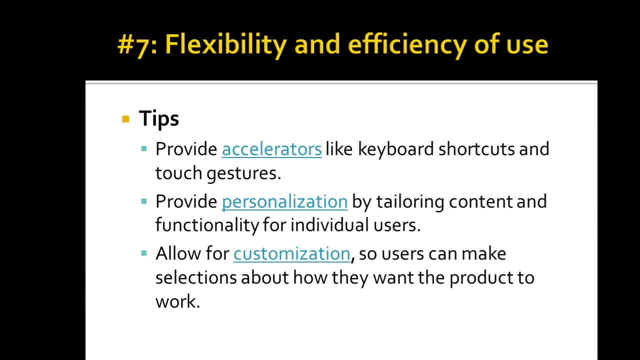 provide accelerators like keyboard shortcuts and touch gestures. provide personalization by tailoring content and functionality for individual users. so something that you can customize or tailor. yes, a little customization. allow for customizations: users can make selections about how they want the product to work. so here's an example. so this is the regular rope for 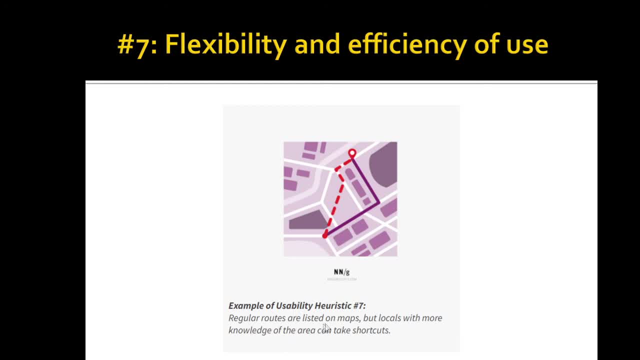 example, this is the regular rope, so regular route for the user to use instead of maps, but locals, so those who know the place, with more knowledge of the area, can take shortcuts. so maybe, instead of doing this, they will be taking this role. so that means that for experts, for 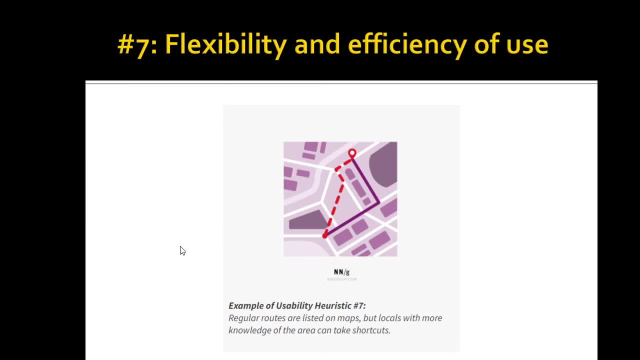 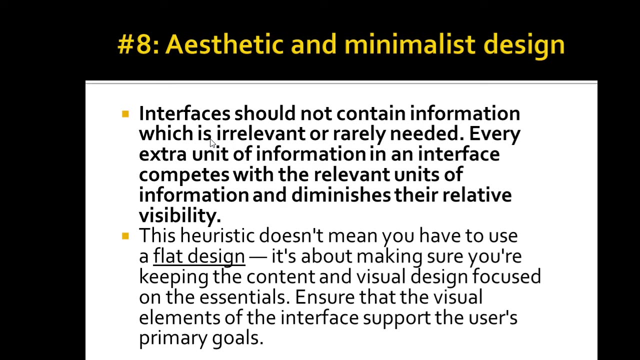 those who are ready experts of the of the software- for example, placing shortcuts- should be convenient to them, and that means that's flexibility and efficiency. number eight: aesthetic and minimalist design interfaces should not contain information which is irrelevant or rarely needed. every extra unit of information in an interface competes with the relevant units of information. 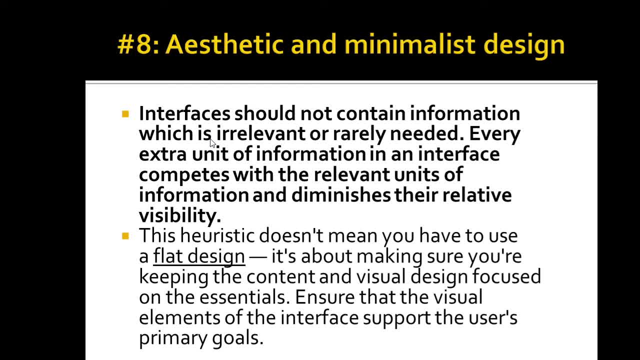 and diminishes their relative visibility. this heuristic doesn't mean you have to use a flat design. it's about making sure you are keeping the content and visual design. focus on the essentials. ensure that the visual element of the interface support the users. primary goals: tips: keep the content and visual design of you. I focus. 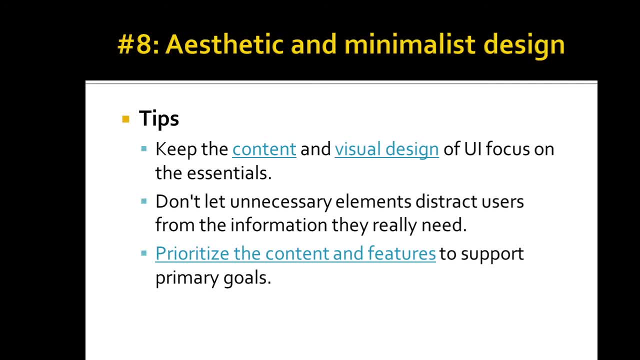 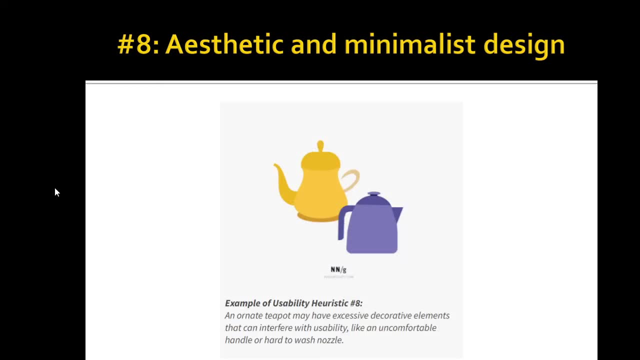 on the essentials. don't let unnecessary element distract users for from the information they really need. prioritize the content and feature to support primary goals. so here's an example: the ornate tipa- this is the only tipa- may have excessive decorative elements that can interfere with. 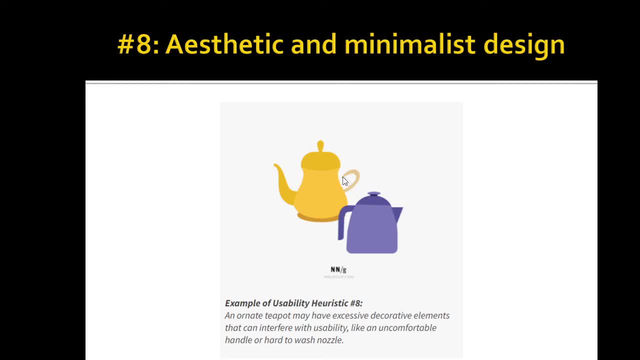 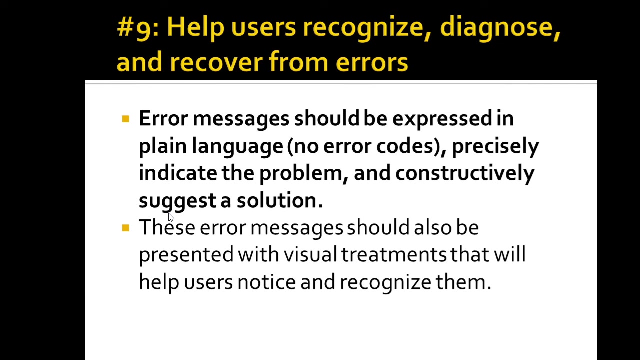 usability, like, for example, and an uncomfortable handle or hard to wash nozzles. the nozzle may be hard to wash, it looks very good, rather than this one, but you notice that the nozzle could be hard to wash and maybe the handle is uncomfortable. number nine help users recognize, diagnose and recover from errors. error messages should. 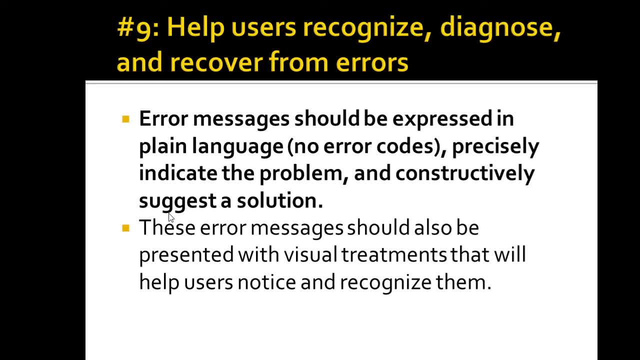 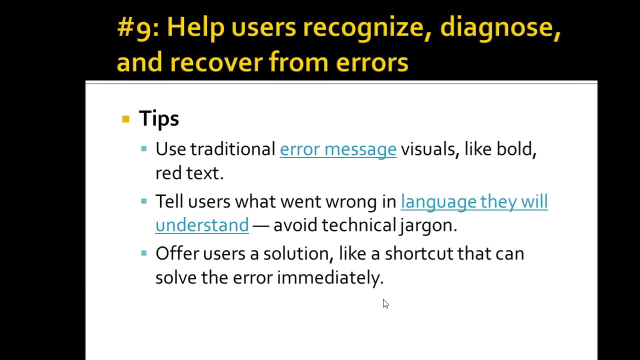 be expressed in plain language. there should be no error codes, so precisely indicate the problem and constructively suggest a solution. this error messages should also be presented with visual treatment that will help users notice and recognize them. so tip, use traditional error message visuals like bold red text, and then tell users what went wrong in a language they will. 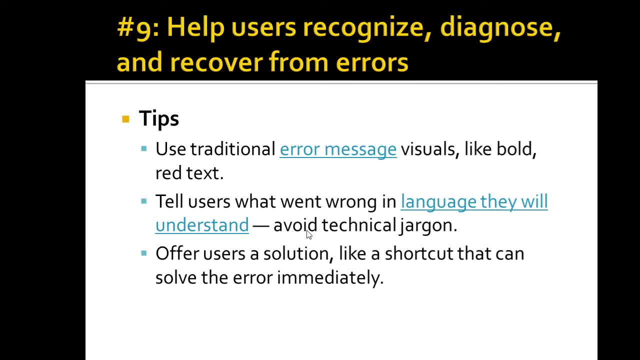 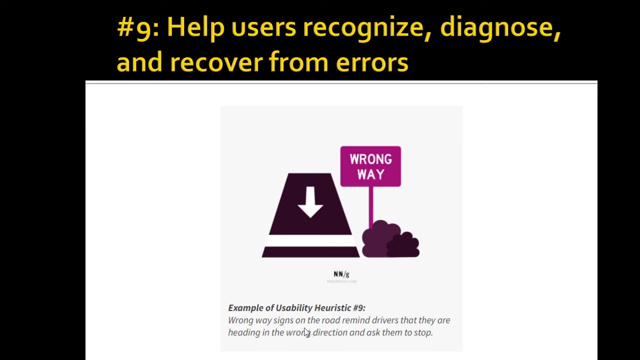 understand and you have to avoid technical jargon and then offer users a solution like a shortcut that can solve the error immediately. so maybe here's a real-world example which is your wrong way. so a wrong way. sign of the road reminds drivers that they are heading. 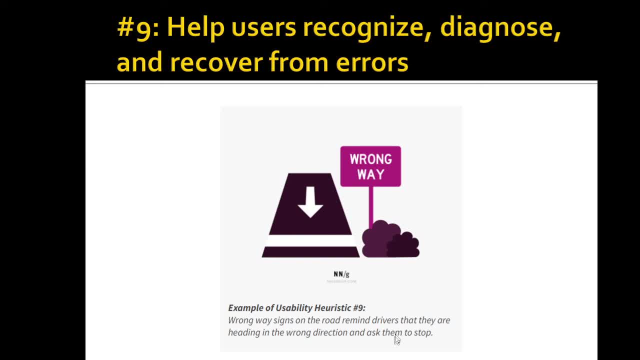 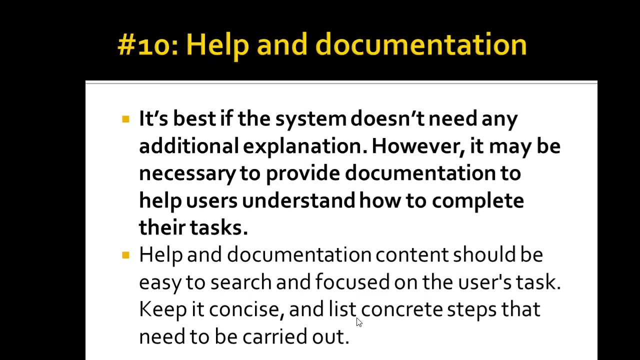 the wrong direction and ask them to stop, and maybe even better if they can place you something, maybe where is the correct way. so this is already a good example of the usability risk. number nine, number ten: help and documentation. it's best if the system doesn't need any additional explanation, however, it may be necessary. 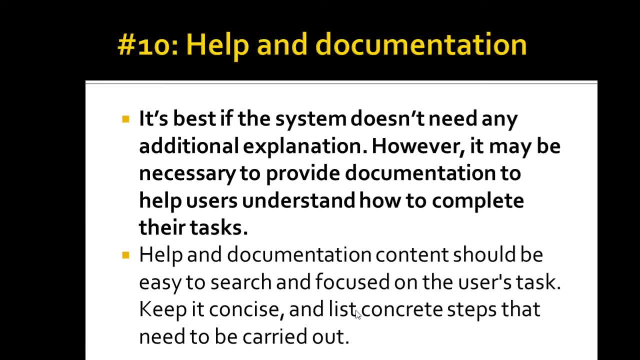 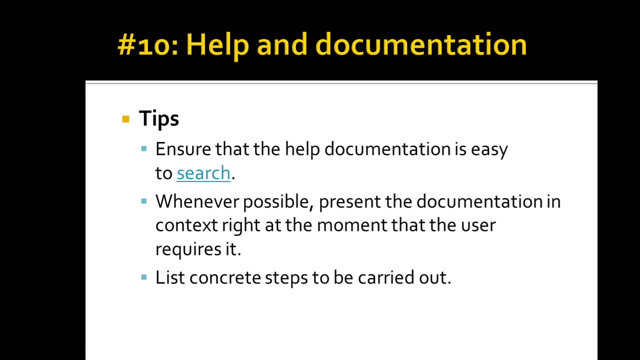 to provide documentation to help users understand how to complete their test. help and documentation content should be easy to search and focus on the user's test, keep it consistent and list concrete steps that need to be carried out. so here are some tips: ensure that the help documentation is easy to search whenever possible. present the documentation in context right. 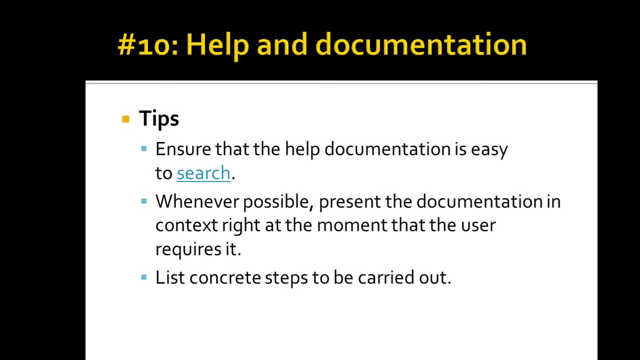 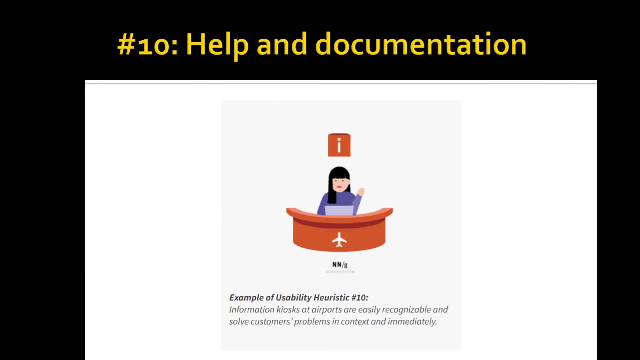 at the moment that the user requires it to list concrete steps to be created. an example of, and see whether or not suas mary in carl brown: toxic energy çokess West putt- i please use this- the skirmishes, which is atinding a 15-hour transfer system in the same area. 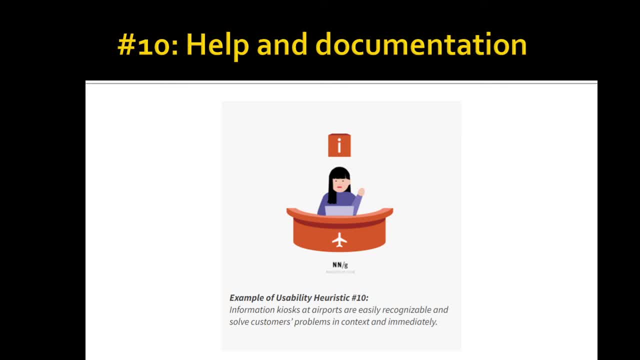 per Louisville. there's firm, safe, go home or valid, may not allow that type in five minutes. more about basic research is absolutely chew about Dthree, everything else. we have so many more steps to look into. recognizable and sold customers problem in context and immediately. so just imagine if you don't have something like this in airports or maybe even schools. 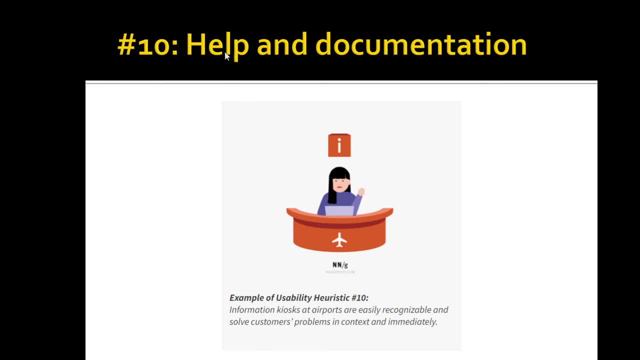 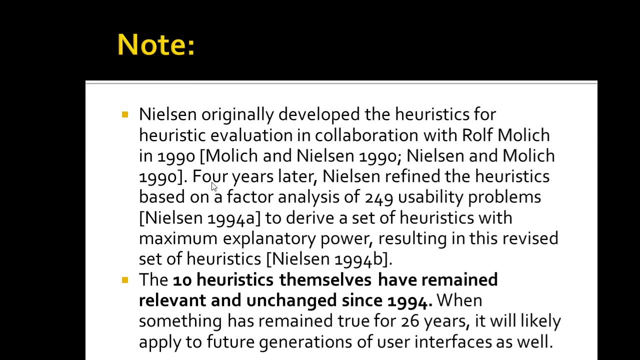 so there should be something like this that are ready to help, maybe students. so just a note to end this video presentation: Nielsen originally developed the heuristics for heuristic evaluation in collaboration with Rolf Mollick in 1990. so that's Mollick and Nielsen 1990. yeah, four years later.